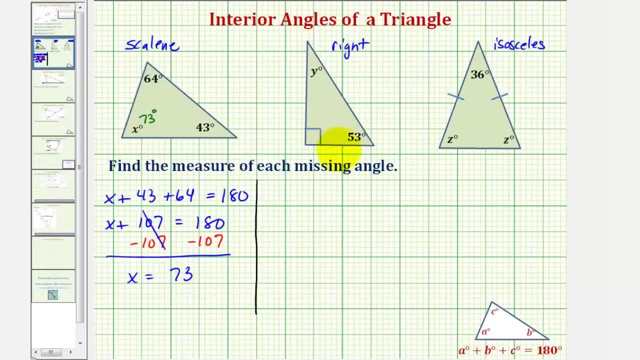 we can set this up a couple ways. The sum of the interior angles must be one hundred eighty degrees, but also the two acute angles of a right triangle are complementary or have a sum of ninety degrees. So let's go ahead and set this up two ways. Let's first use the fact that y 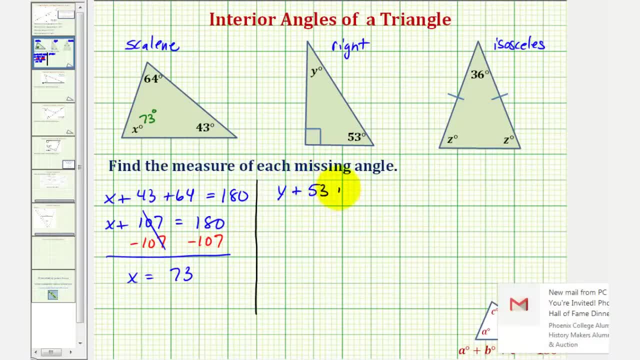 plus fifty-three plus ninety must equal one hundred eighty. So we have y plus this would be: one hundred forty-three equals one hundred eighty. Subtract one hundred forty-three on both sides and we have: y equals one hundred eighty minus one hundred forty-three is thirty-seven. 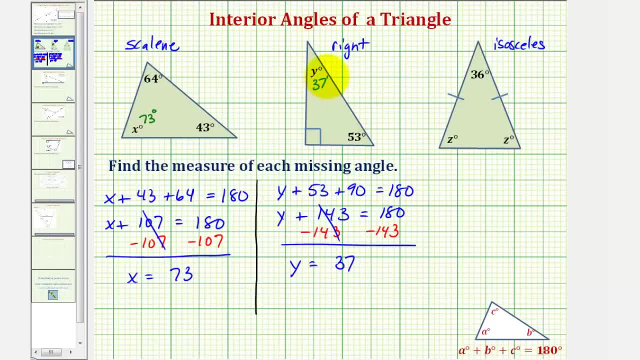 Therefore, the measure of the missing angle is thirty-seven degrees. The other option would be to recognize that y plus fifty-three must equal ninety degrees, because these two angles are complementary. Subtracting fifty-three on both sides, we get the same result: y equals thirty-seven. And then, finally, for our Sausalese triangle, 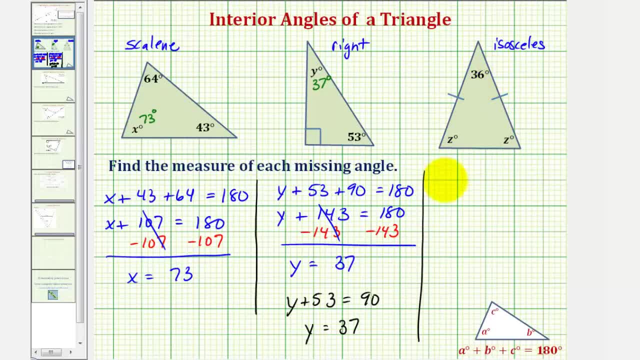 our equation would be: z plus z plus thirty-six equals one hundred eighty Z plus z would be two z. So here we have a two-step equation to solve. We'd first subtract thirty-six on both sides. This would give us two z equals. 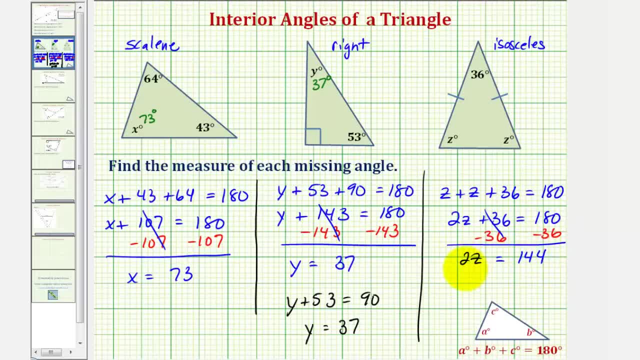 one hundred forty-four. And now to solve for z, we divide both sides by two, So we have z equals one hundred forty-four, divided by two equals seventy-two. And therefore the two missing angles, which are equal in measure, both measure seventy-two degrees. I hope you found this helpful.